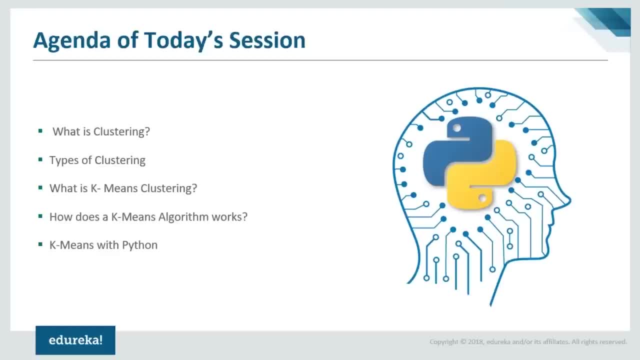 what is clustering, types of clustering? What exactly is k-means clustering? How does k-means algorithm work? And then, finally, we'll implement k-means using python. Yeah, one more thing. this implementation part would be divided into two different parts. right in the first part, We'll 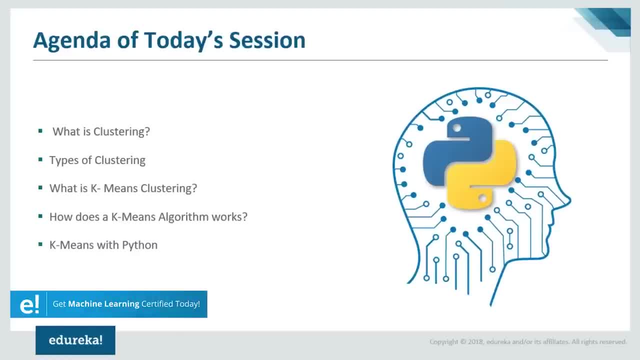 learn how to implement k-means using python from the scratch, I like, and in the next part we'll be using python on inbuilt library for implementing k-means algorithm, All right, and then finally, we'll compare output of them, since you guys know that the main topic of discussion for this particular 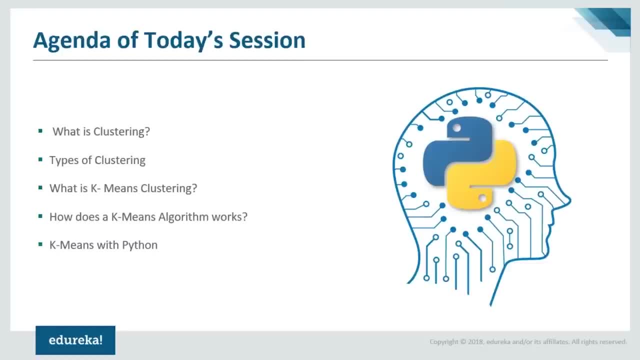 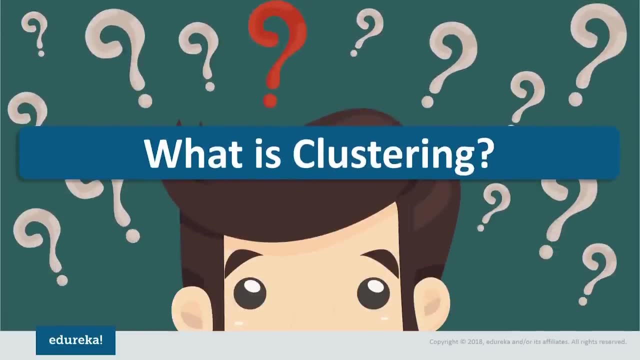 session is on k-means clustering, But before I dive deep into it, let me ask you a question: Do you guys know what exactly is clustering? because it's very important that you know what clustering before we drill down to see what exactly k-means clustering is. So any answer, anyone? 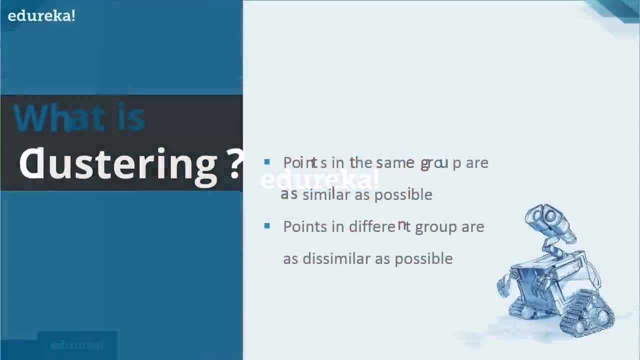 Okay, just let me tell. so what is clustering in simple words? If you want, clustering is nothing but creating different groups. the groups consist of similar element. If you want a definition kind of thing, then you can define clustering as a process of dividing the data sets into groups consisting of similar data points, the point within one cluster. 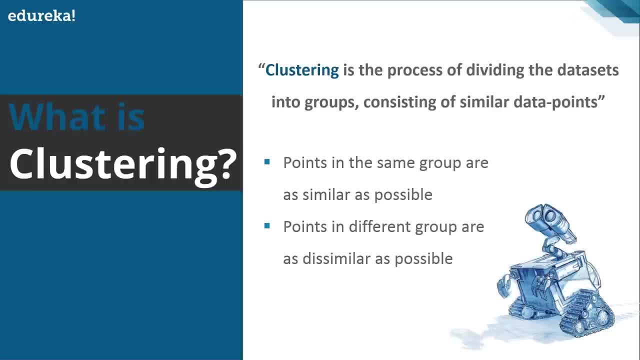 are as similar as possible, Whereas the point belonging to other cluster are completely different from the points in the first cluster. All right, and here's one more thing. clustering is often referred as an unsupervised learning technique. Now you would ask that what is the use of clustering? 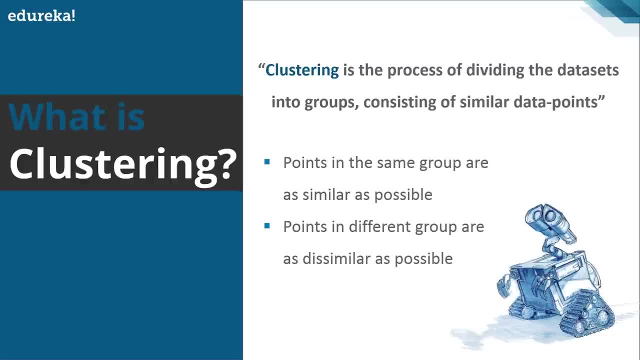 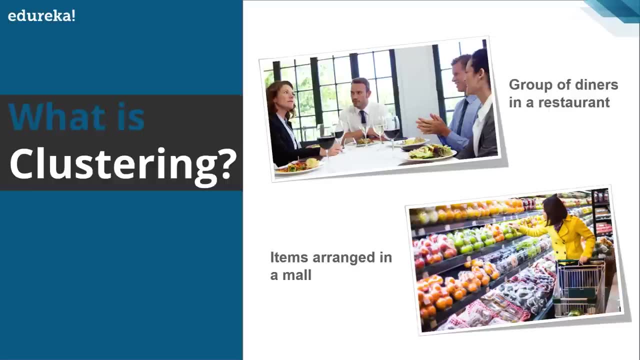 or where is it All right? so it is very important to know, so where it is used. So let's understand clustering with an analogy. So in my introduction part, as I said that a group of diners sitting in a restaurant is an example of clustering, Let me tell you how you can connect it with the definition of clustering. 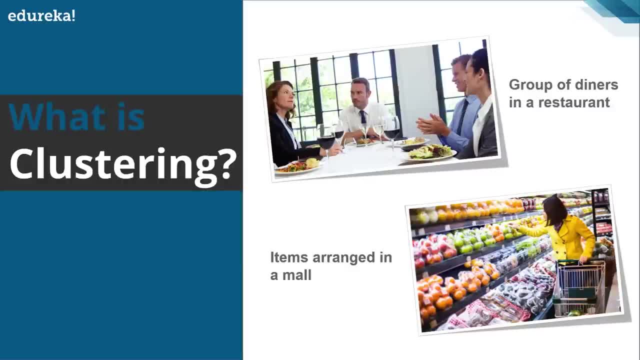 All right. suppose there are two tables in a restaurant, all right, table t1 and table t2. the group of people sitting on the table t1: they might be related to each other, right? They may be a group of family member, They may be a group of colleagues or anything. right, Even the people sitting on the 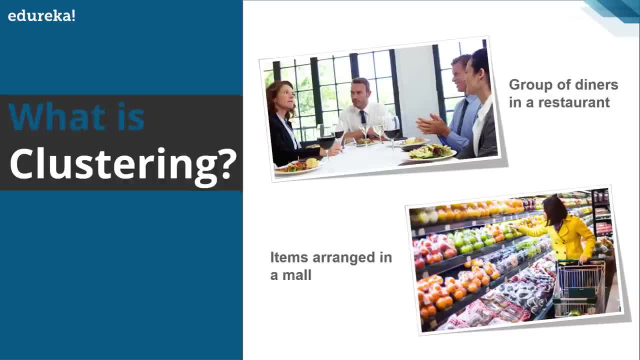 table t2. even they are connected with each other, but only among the people sitting on table t2, right, But when it comes to comparing the people sitting on table t1 to the people sitting on t2, you'll see that they are entirely different, that not at all related with each other. All right, 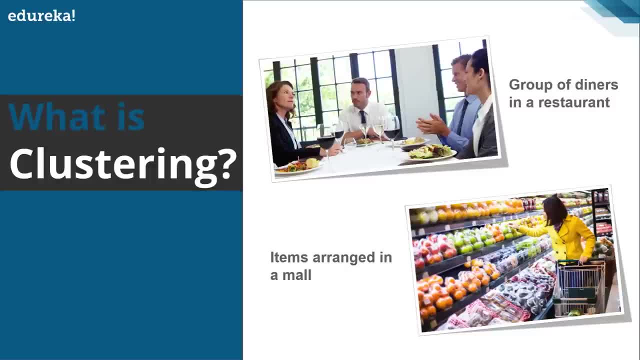 so this clustering is also done in the same way. What is it? It's that the data points within one cluster is entirely different from the data point of the other cluster. All right, and all the points within the same cluster are either same or are related to each other. All right. next was the items. 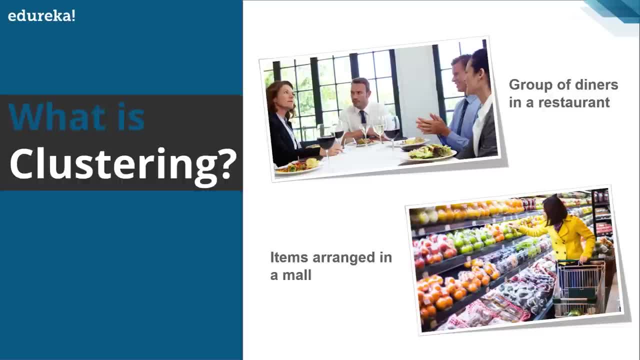 arranged in a mall. Remember, when you visit Walmart or a retail store, you would find that similar items are grouped together for you. It's not like the items are just placed anywhere mixed with each other, like the fruits and vegetable section. You won't find that apples and oranges are. 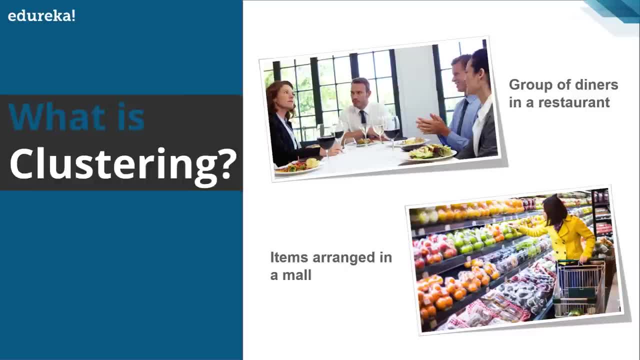 mixed with each other and placed on the shelf right. So what they do? they create groups and cluster of items for you so that you can easily shop and find your things from it. All right, It's like same variety of apples are placed in one place, while the other varieties of apples are placed in another. 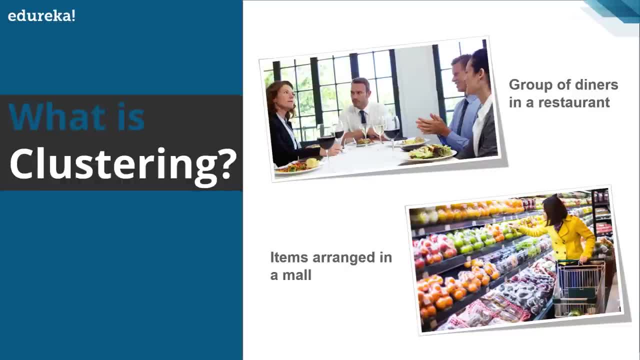 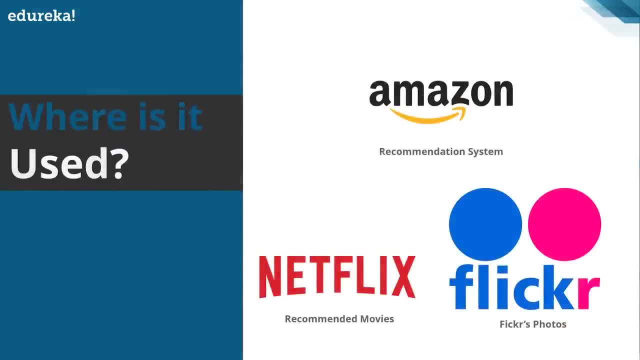 you won't see the Mix, Mix Match of red and green apple, right? So when this is clustering, all right, so let's move ahead. Now the next question comes: where is it used? So let's see, one by one, flicker maps of photo and other map sites. uses clustering to reduce the number of markers. 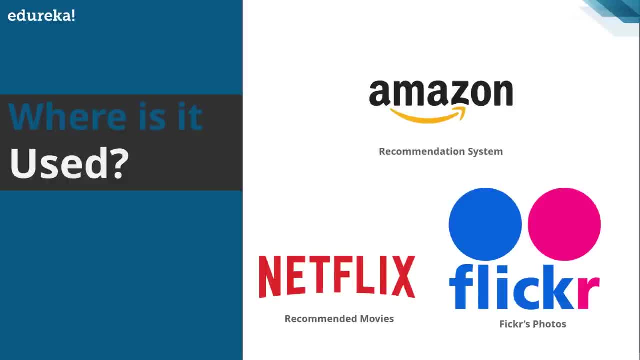 on a map. Even the Amazon is using the popular recommendation system, which is using the clustering to show you the recommended list of product according to your past purchase history. And, yes, even the Netflix: it recommends you the movies based on your watch history. right, 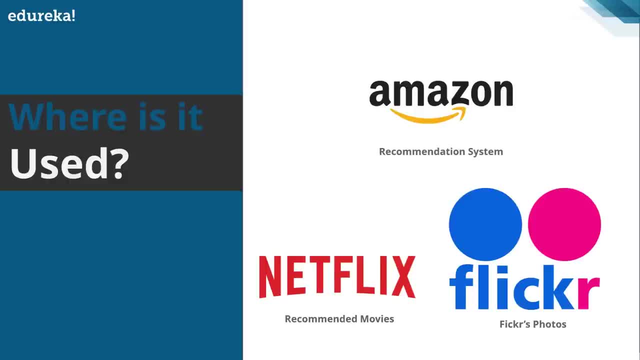 Whatever you have watched, it will show you some similar movies related to it. All right, So how do you think these recommended list are generated? Well, all the concept lies behind this clustering I like. well, in general, you can say that clustering can be used to segment the customers. 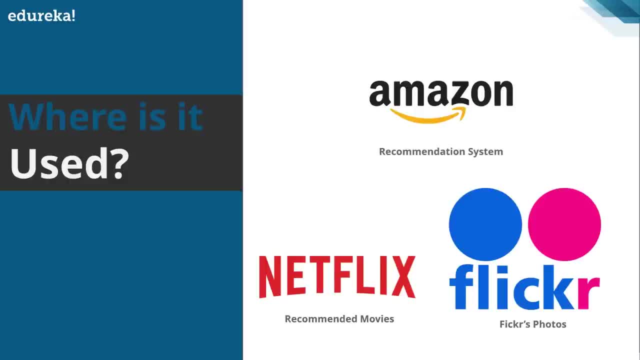 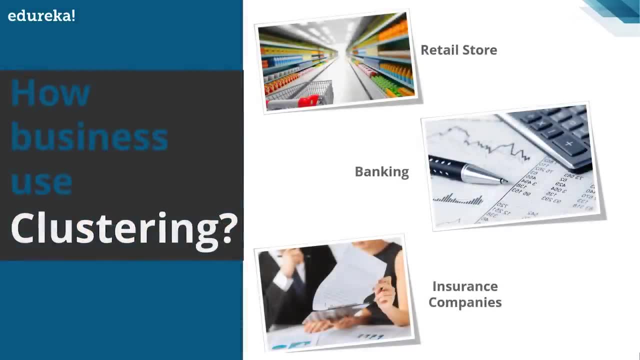 or Market. in the marketing. It can be used by the social Network site and marketing new groups based on users data. All right, so let's move on and see how business is using clustering. will clustering can help the business to manage their data better? Generally, they use clustering for image segmentation. 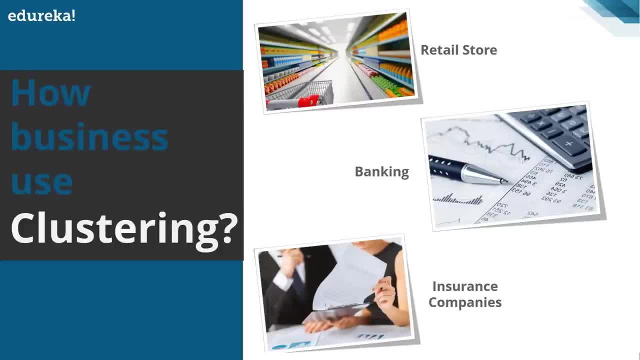 Grouping web pages, market segmentation and information retrieval. For example, in a retail business, the data clustering helps in analyzing the customer shopping behavior, sales campaigns and customer retention. in case of insurance company, a clustering is deployed in a field of fraud detection, risk factor identification and customer retention efforts, while in the case 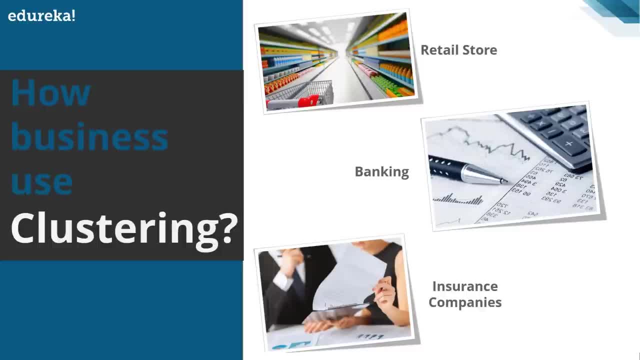 of banking sector. you can use it for customer segmentation, credit scoring and analyzing customer profitability. All right, so this is how the clustering is used in Various business. All right, let's move ahead. Let's see What are the different types of clustering. 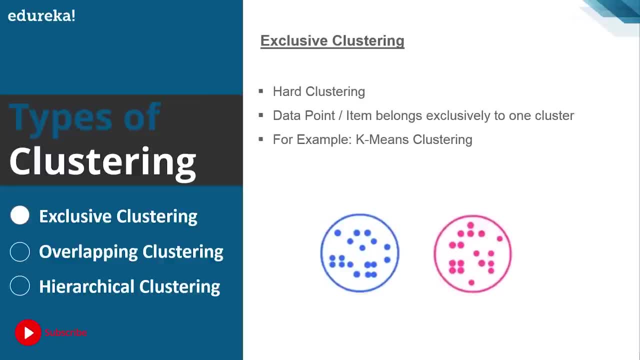 Well, we have mainly three different types of clustering: exclusive clustering, overlapping clustering and hierarchical clustering. Let's start with exclusive clustering. Well, this exclusive clustering is a hard clustering in which the data points or the items exclusively belongs to one cluster. an example of such clustering can be a canines clustering and the example shown below you can see. 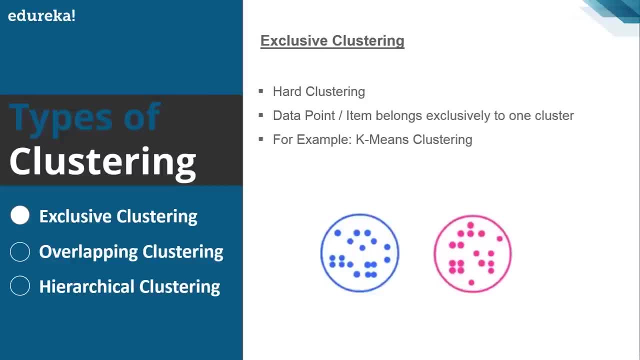 that all the blue data points lie within the blue cluster and all the pink Data points they lie within the pink cluster. Both these clusters are entirely different from each other. They are not at all related with each other. All right, so this is how it's- a example of exclusive clustering. next comes the overlapping. 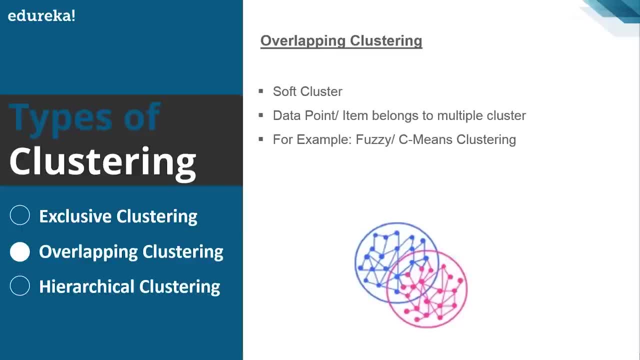 clustering. Well, this overlapping clustering is a soft cluster in which the data points or the item belong to multiple cluster. an example of such clustering can be fuzzy, or see means clustering. even in the diagram You can see that some of the blue data points are overlapping with the pink data points. 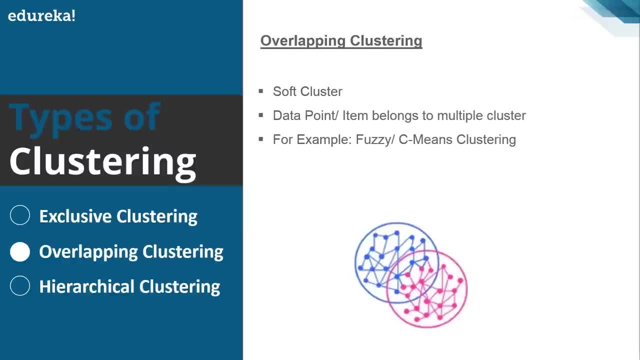 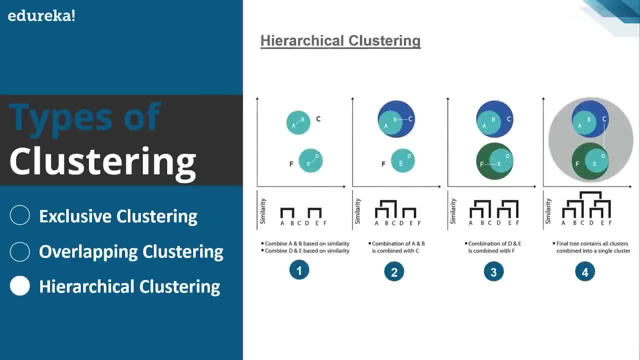 All right. So this is what happens in a c-means clustering of the fuzzy clustering. There's what a overlapping clustering is. All right, fine. next comes the hierarchical clustering. Well, let's understand hierarchical clustering with this example. Let's consider case one, for instance. consider that we have six data points: a, b, c, d. 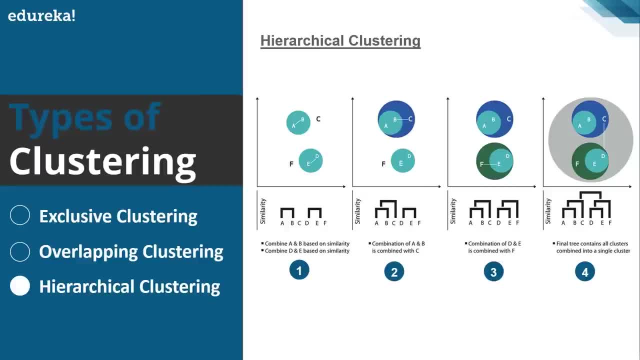 and e, out of which a and b are similar and d and e are similar. All right. So in the first case, what we are doing, we are combining a and b based on some similarity and we are combining d and e even based on their similarity. 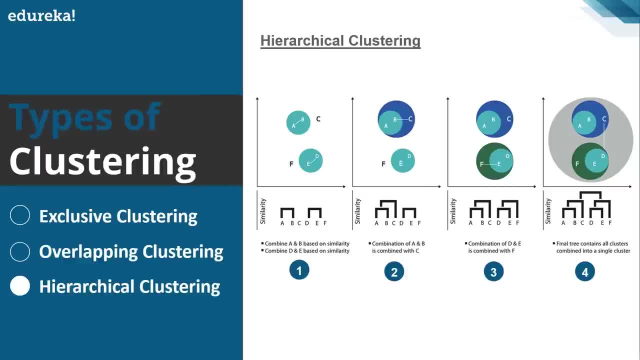 All right. in the next part, What do we see? that the combination of a and b is quite similar to C. So we are combining the combination of a and b with the C, All right. and similarly, in the third part, We see that the combination of d and e, it is quite similar to F. 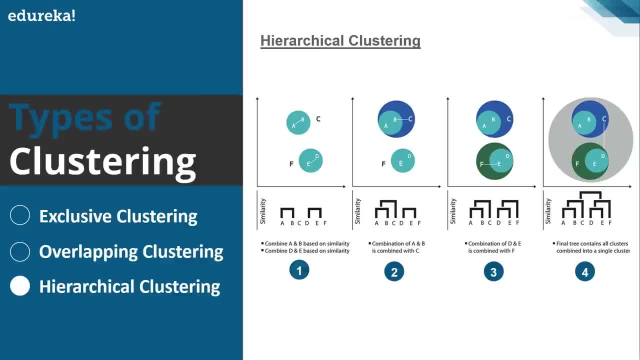 So we are combining the combination of d and e with F. Okay, and the final fourth part. We see that the final tree contains all the cluster combined within a single cluster, as the combination of a, b, C is quite similar with the combination of d, e, F. 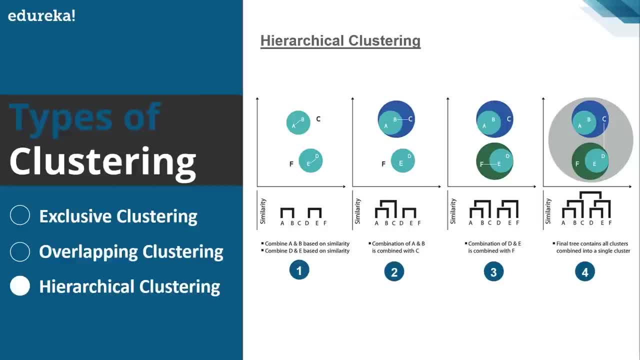 Okay, so the final tree contains all the cluster combined into a single cluster. All right, So this is what a hierarchical clustering is and how it works. Okay, an example of hierarchical clustering can be a dendrogram. All right, till now we have covered about what is clustering. 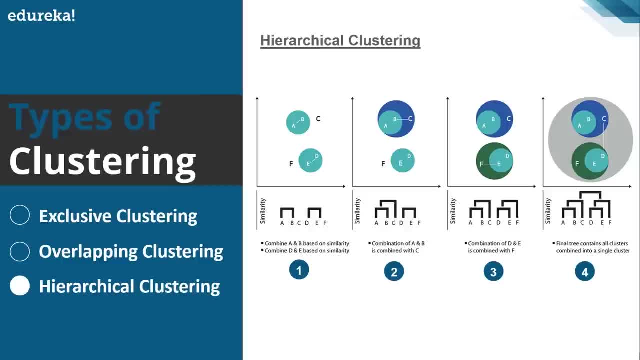 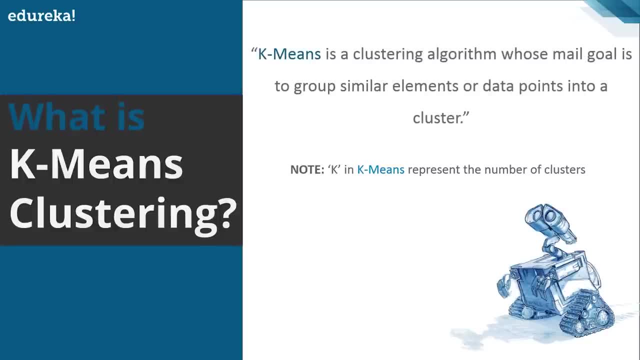 where it is used, how the business is using clustering and what are the different types of clustering available. All right now, since our main focus would be on k-means clustering, So let's focus on that. So, what is k-means clustering? Well, k-means is a clustering algorithm whose main goal 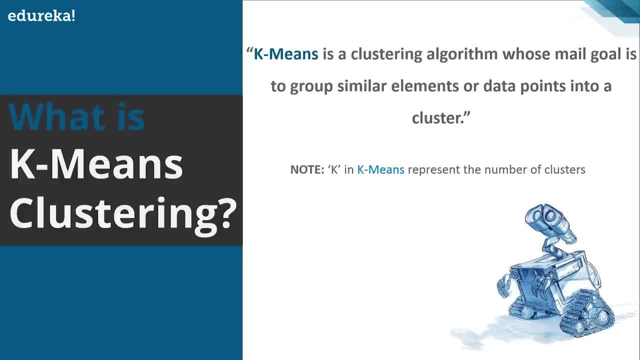 is to find the groups in the data. The number of groups or cluster, is represented by K. the algorithm then runs iteratively to assign each data points to one of the K groups, based on the features that are already provided. Okay, Now let's understand this. k-means clustering. with an analogy. 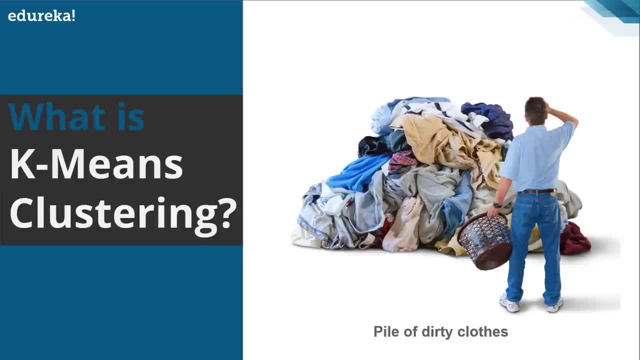 Suppose that you are shifted to your hostel and you don't know how to wash your clothes. You have to do your laundry on your own, All right. So at the end of the month you see that you have collected a big pile of clothes for you. 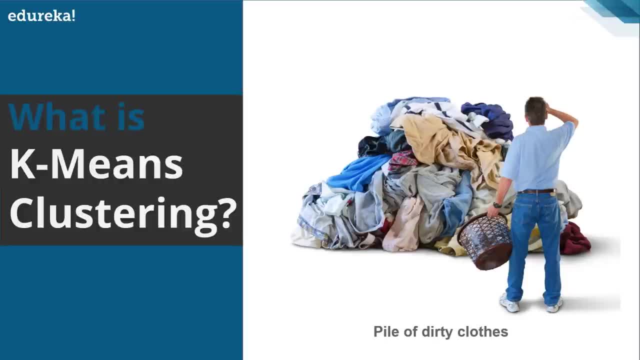 and they are waiting for you to wash them. So how will you do that? So what you did initially: you call your mother. you asked her how to wash these clothes. She said that their specification for each variety of clothes. Okay, some are washed in hot water, some in cold, some can be. 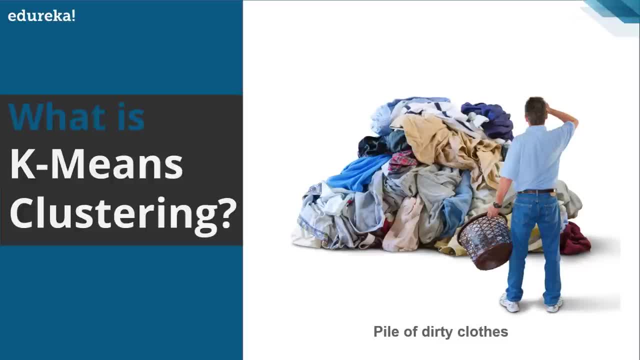 put in the dryer, some need air drying and so on. They are various specification for various clothes. All right, to make this a clustering scenario, Let's assume that your mother asked you to divide into three parts. Okay, She asked you to pick. 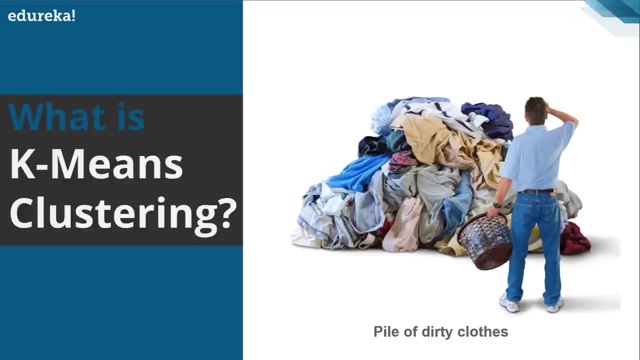 Three different items of clothes at random, and that will be the starting point for those three separate clusters. And then again you have to go through that massive initial cluster and look at each item of clothing in turn. Now, at this point of time, you have to compare the attributes. 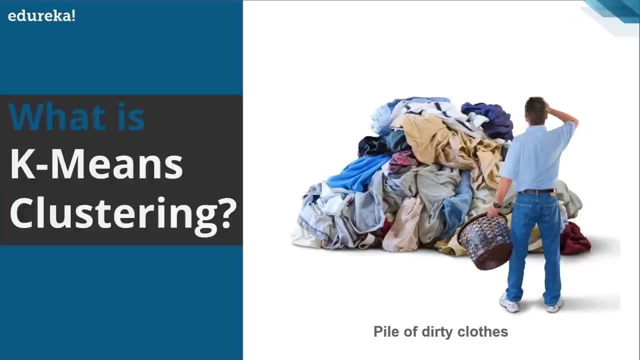 such as water temperature, drying temperature, color, with each of the three starting item and then place the new item into the best cluster or the best pile. Okay, So what do you think is the definition of a best cluster or a best pile? Well, it is not based on a whole cluster. 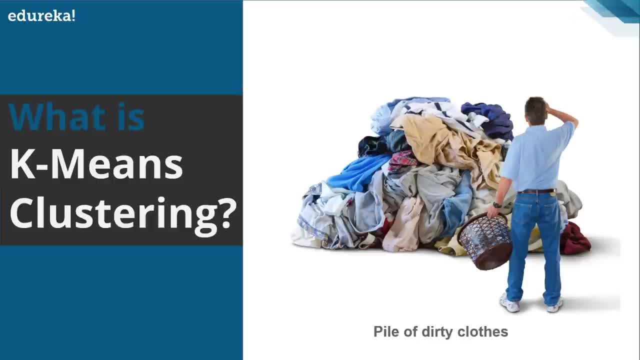 It purely rely on the starting point. Technically, that starting item is known as centroid, but don't worry about that, We'll get to know about that later. These items won't be identical, So pick the best match if you want to be really detailed. 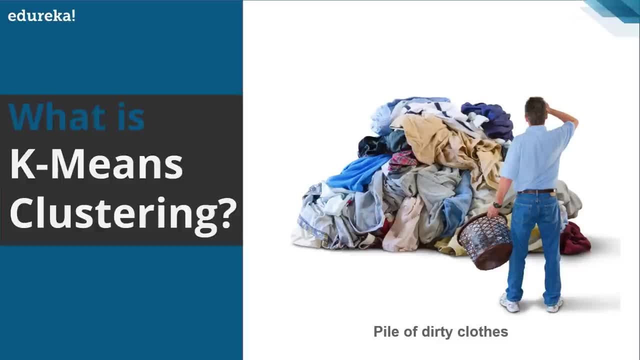 about this. So what you have to do, you ask to place each item closer to or farther away from the starting item, based on how similar they are. that is, you can say that the more similar is the item, the more closer it will be to the starting point. 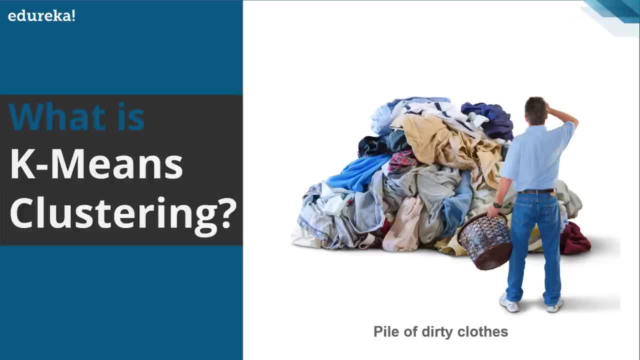 Okay, Now you have got three Different cluster, which means you are ready to use the washing machine, but not so fast. We are just getting started. Well, there's a very iterative process and the next step would be to determine the new centroid. 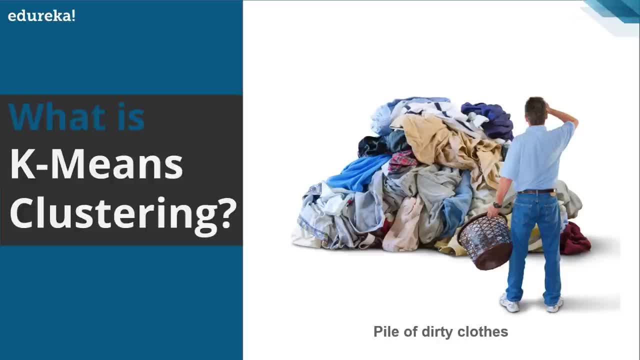 for each of those pile or each of those cluster and repeat the process. those new centers would be calculated and may not correspond to an actual item of clothing and we really don't know if these three clusters are optimal number. So once you have completed the iteration with three cluster, 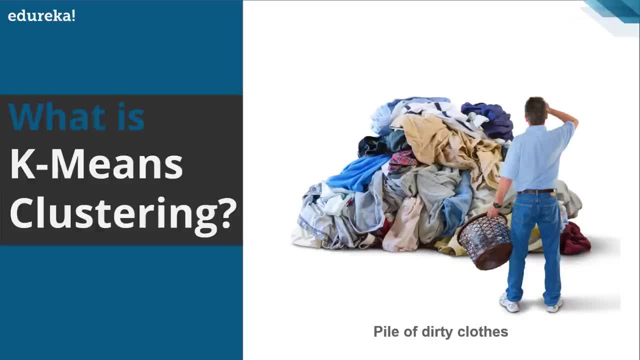 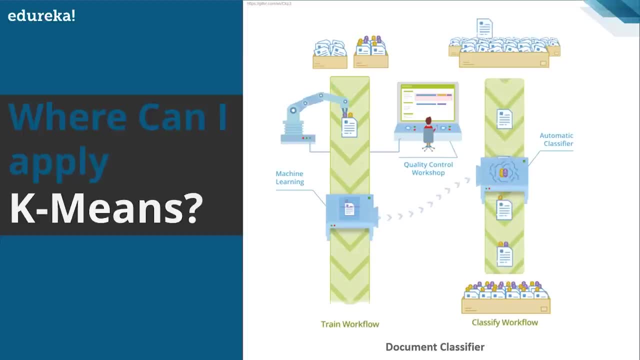 you should go and try with four, five and more. Now there's what k-means algorithm was. don't worry, We'll see more details about it, But first let's see where you can apply the k-means algorithm. The k-means algorithm can be applied to a numeric. 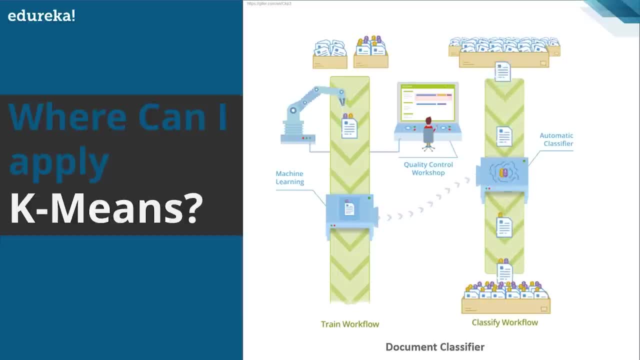 or continuous data with smaller number of dimension. It can be applied to any scenario where you want to make groups of similar things from randomly distributed collection of things, For example, document classification, where you can create the clusters of document and multiple categories based on tags, topics. 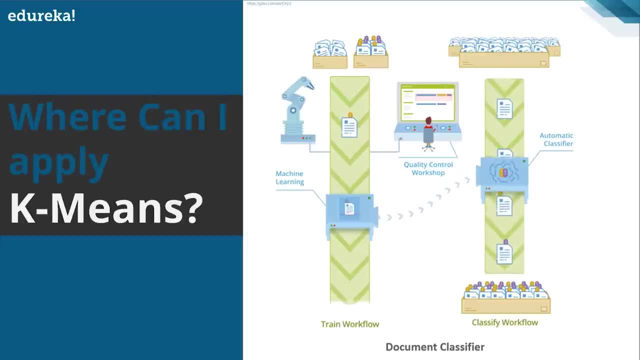 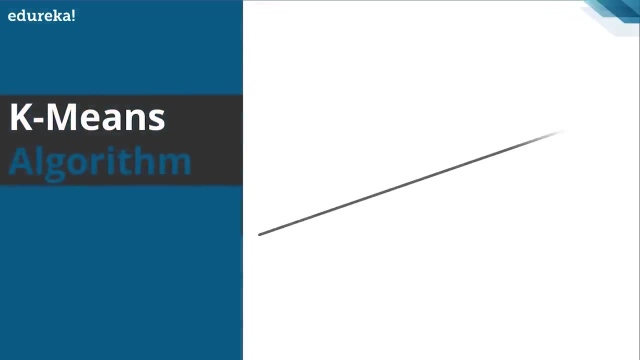 and contents of the document. This is a very standard classification problem and k-means algorithm is one of the highly suitable algorithm for this purpose. Now let's proceed and understand about k-means algorithm in depth. Imagine you have some data and your task is to plot the data points on the graph. 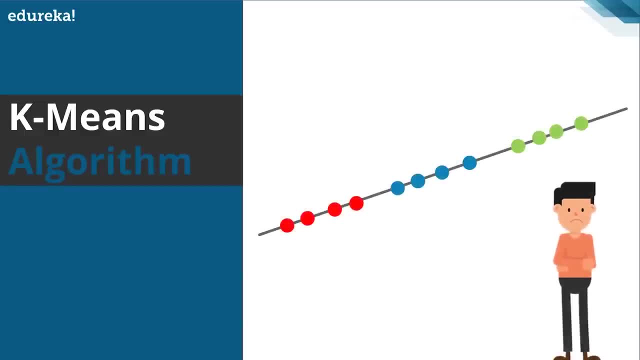 and divide the points into three different cluster. Now these three cluster may represent three different categories of, suppose, bikes. in the data set It might be a cruise sports or touring bike. Okay, so in this case you can see the exact data points within each cluster. 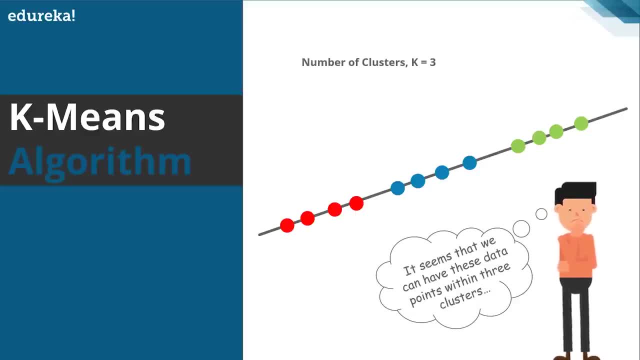 but rather than just relying to our eye, let's see if our computer can show us the same result or not. That is three clusters. in order to perform this, I'll be using the k-means clustering. Now let's suppose there's a unclustered data. 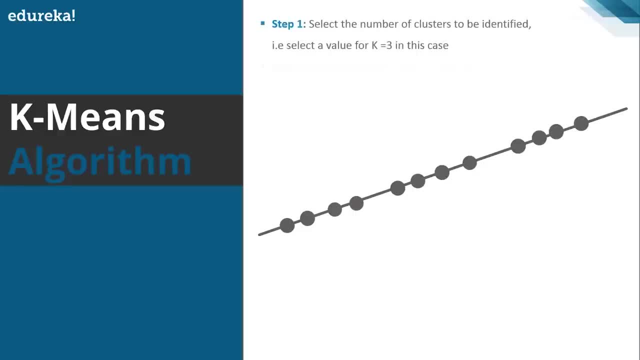 So, to start with, at step one, you will select the number of cluster you want to identify in your data. Let me tell you a fact: that this k in k-means is nothing but the total number of clusters you want. suppose of k equals 3. 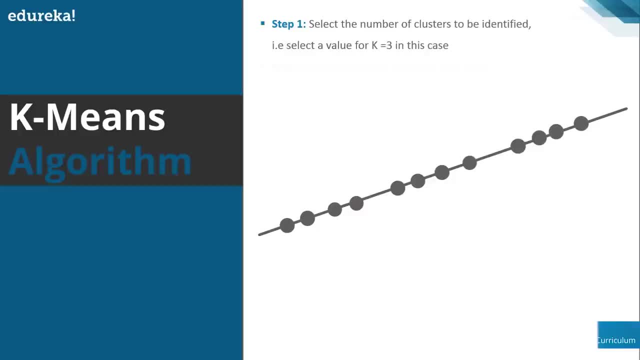 then total number of cluster is also 3.. Okay, So in this case it's k equal 3. as it is mentioned already that we want to create three clusters, There's also a very cool way to select the number of K, but we'll discuss about it later in this session. 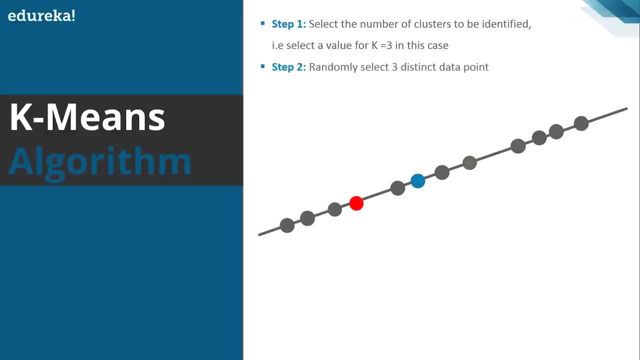 Okay, and step 2: what we do? we randomly select three distinct data points. So these are the initial three cluster consisting of just one single data point. Okay, these three points are nothing, but we are assuming that they are the centroid of each cluster. 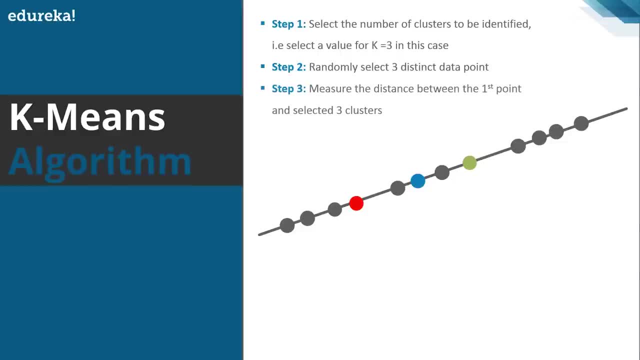 Okay, Now, as a step 3, what we'll do will measure the distance between the first point and the three clusters. So that shows the distance from the first point to the red cluster. next, It shows the distance from the first point to the blue cluster. 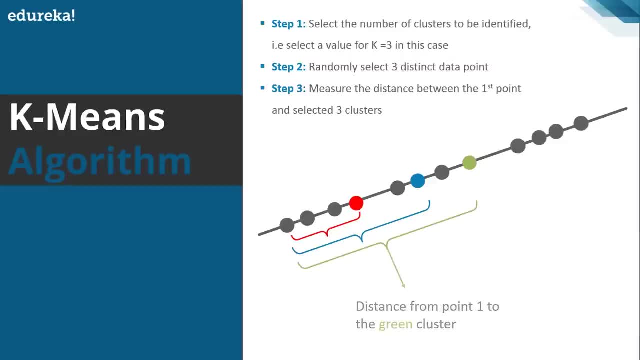 and this: it shows the distance from the first point to the green cluster, I like, moving on to step 4.. What we'll do will assign the first point and add the first point to the nearest cluster, since, in this case, the nearest one is red. 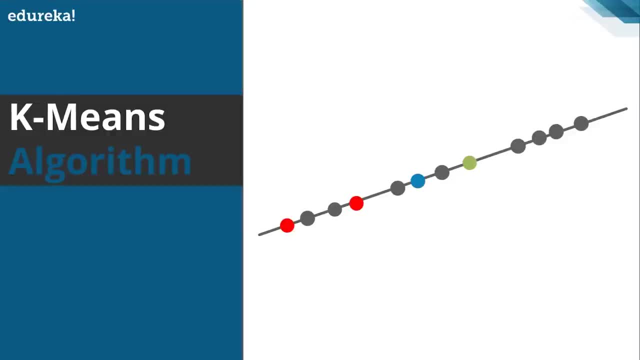 So the first point will be added to the red cluster. fine, as a step. 5 will calculate the mean for the red cluster, including the new point which is recently added to the cluster. So the mean value in this case lies somewhere here in between the two points within the red cluster. 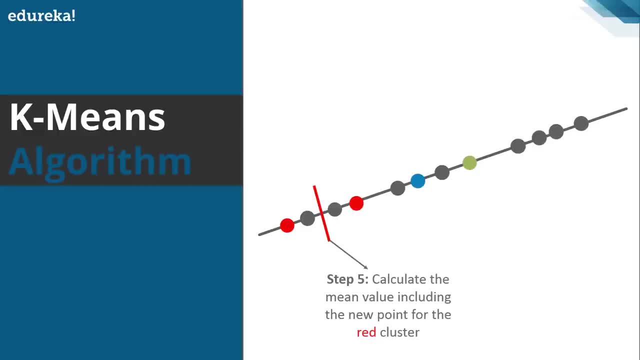 Okay, Now we are done with first point. We know that the first point lies within the red cluster. Now let's figure out the cluster of the second point, or in other words, to which cluster does the second point belongs to. well, to do this, 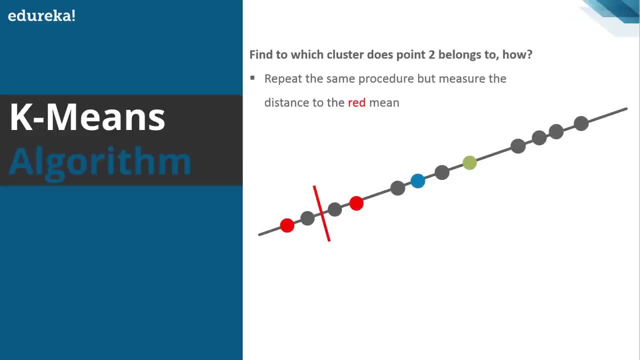 You can use the same procedure you use for the first point. It's just that will now measure the distance of second point from the red mean. So here is the different distance of second point to different red, blue and green clusters. Once you are done with measuring, assign the second point. 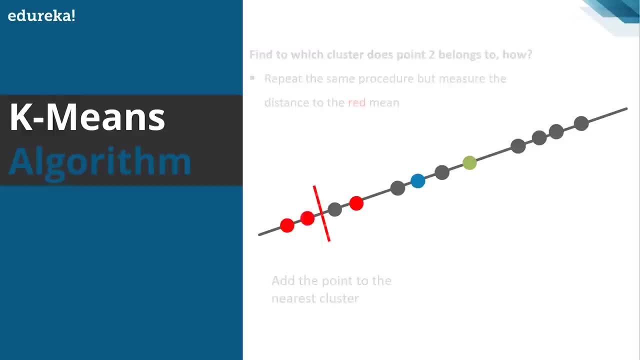 to the nearest cluster, which is again the red cluster. All right. next we'll use this new point to calculate the mean within the red cluster. as you can see, this new mean is shifted to the left just a little bit right. So now we know about our second point as well. 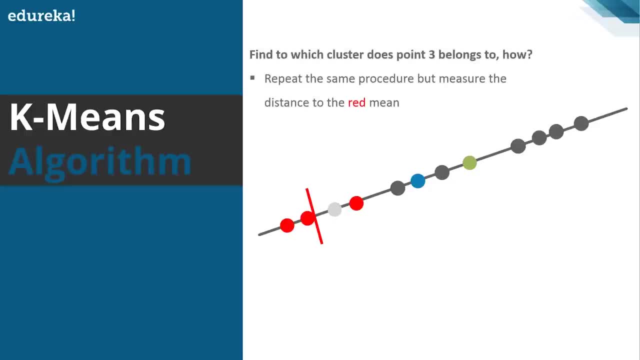 Even it lies within the red cluster. Now let's see and find out which cluster does our third point belongs to. so what we need to do again: measure the distance, assign the point to the nearest cluster and then finally calculate the new mean for the red cluster. 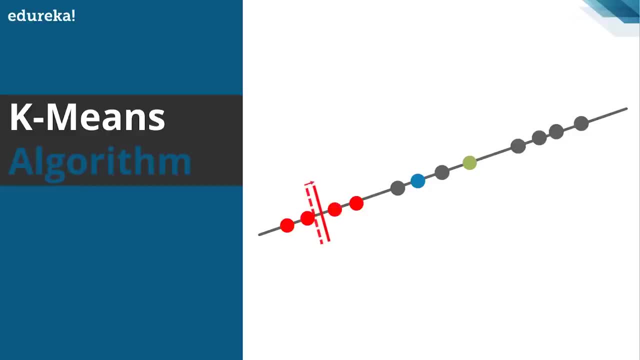 as this particular third point. even this belongs to the red cluster. All right, Now let's move on to see which point is. the fifth point belongs to again follow the same method, measure the distance, assign the cluster and once again calculate the new mean. for this case, for fifth point. 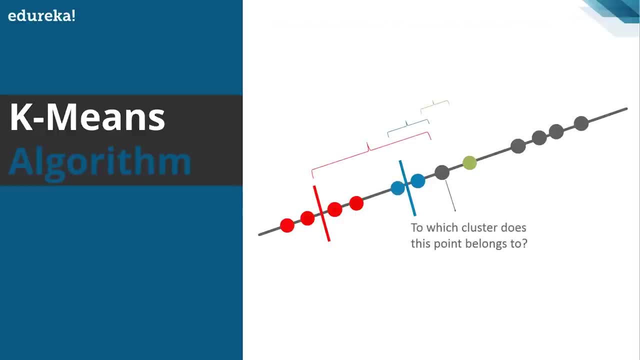 You can see that it belongs to the blue cluster and it is a blue point. Okay, Now let's find out to which of the cluster does this point belongs to again measure the distance, assign the cluster, calculate the new cluster, mean the rest of these. 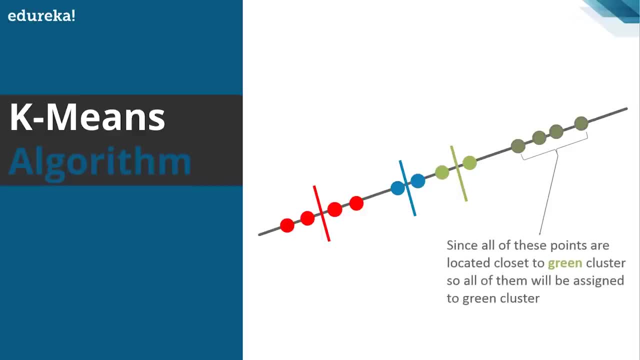 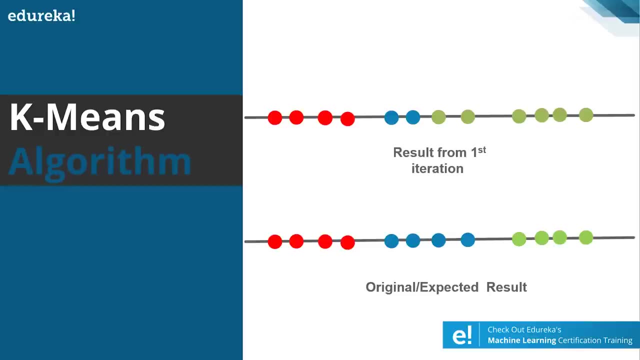 points will always be closest to the green, So all of these will fall under the green cluster. That's time We compare our result to the original one. Oh what this k-means. clustering algorithm, or the machine, is giving a very poor result compared. 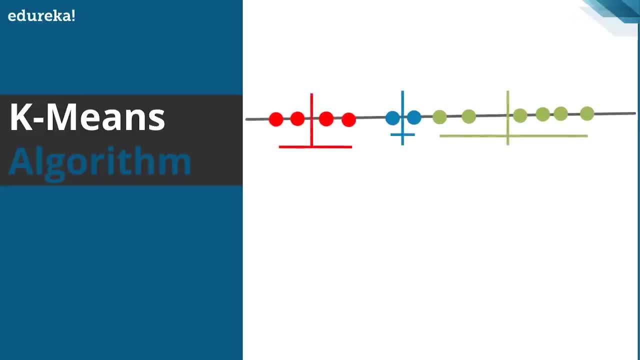 to what we did by I will. you can always check the quality of the cluster data just by adding up the variance within each cluster. So there's the sum total of variance within the three clusters. Well, there's a fact that k-means clustering cannot see. 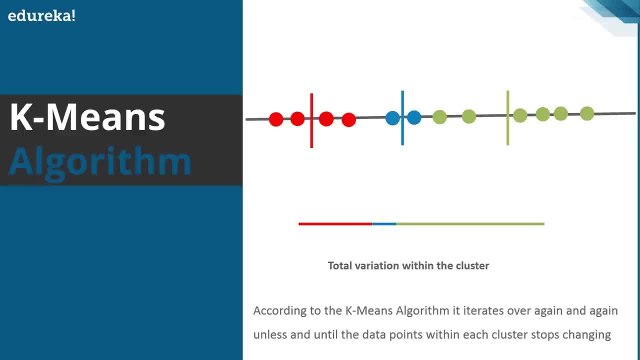 which one of them is the best clustering. but what it does? It keeps a track of these clusters and their total variance and repeat the same steps from the scratch, but with different starting point. So let's see once again. we are here at the beginning to choose three random points. 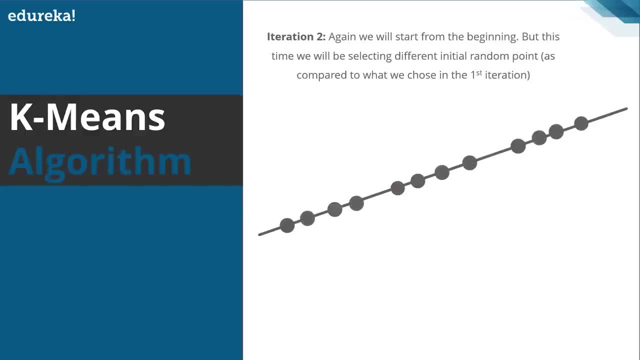 but, yeah, make sure that these three random points are completely different from those random points which we had selected in the very beginning. Okay, so, algorithm what it does? it picks three initial cluster and then it adds the remaining point to the cluster, having the nearest mean- again recalculating. 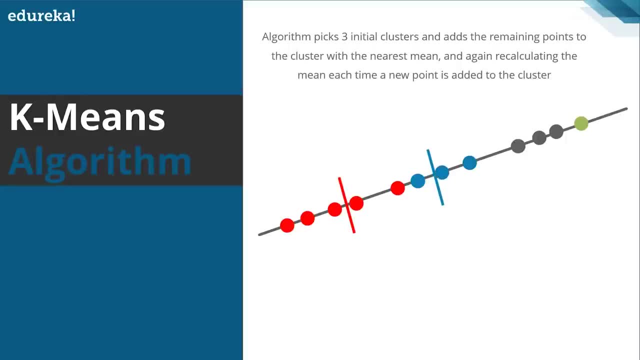 the mean each time a new point is added to the cluster. Now, once we have the cluster data, will calculate the sum of variation within each cluster and again repeat the same steps again and again: pick three initial cluster, cluster, the remaining point and finally take the sum. 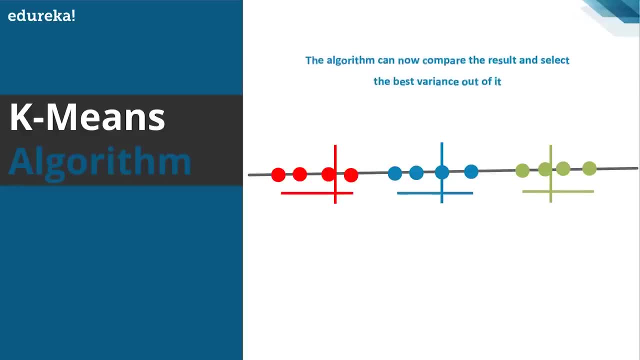 of variation within each cluster. now, at this point our algorithm knows that is the best clustering so far as it has the lowest sum of variation. but even now the algorithm is not completely sure of the cluster, So it will repeat itself and check for a few more cluster. 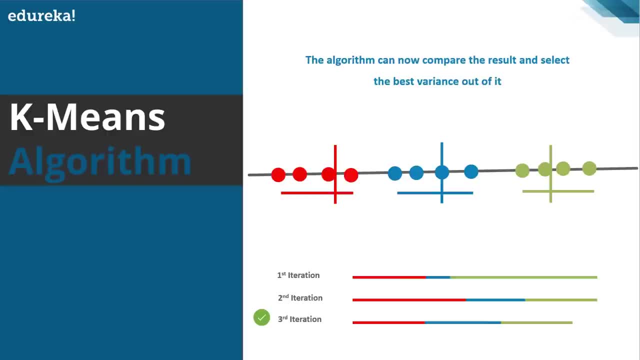 Now you might be wondering when this algorithm would end. Well, it depends on how many iteration you want to perform. It would do as many as you wanted to do. Suppose I say I want to perform 20 iteration, So the machine will iterate 20 times. 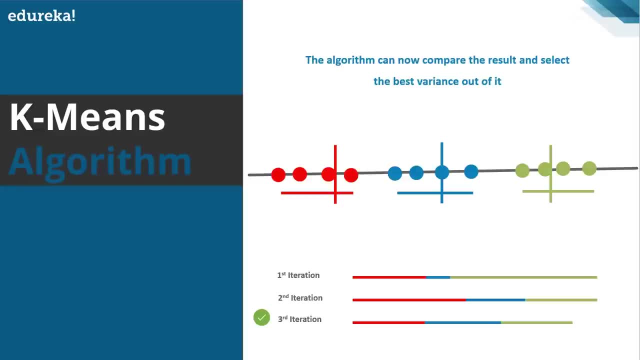 and then finally return the result. It's not like if you perform 20 iteration, you will be getting 20 different cluster. It's just that it will execute 20 times even though the result is same. by same result I mean that the cluster created would stop changing. 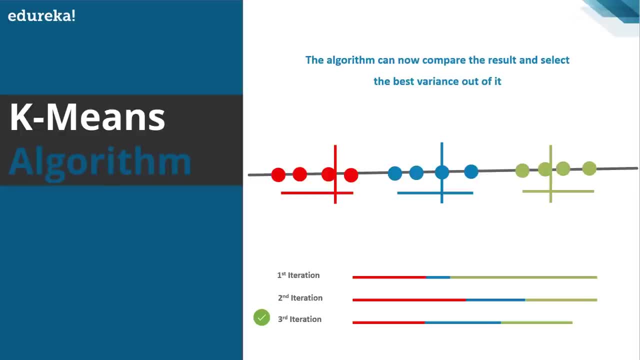 after a few iterations, All right. when manually calculating, we generally stop the calculation when we get the same result consecutively, as we want to get short of the result, even though you repeat, you would get the same result. Okay, Now what if we have a 2D data plotted on a graph? 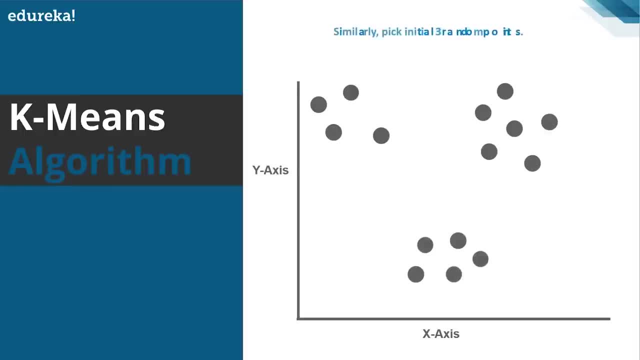 with X and Y axis. So even for this case, we'll start with picking up three random point which will be their centroid, But in this case we'll use the Euclidean distance to find the distance between the two points. in case of 2D. 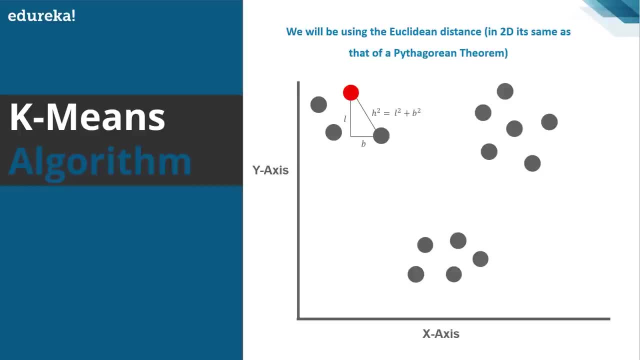 This Euclidean distance is same as that of a Pythagorean theorem like that is H square equal L square plus B square, where H is the hypotenuse, L is the length or the height and B is the base. Okay then, just like before, you will assign the point. 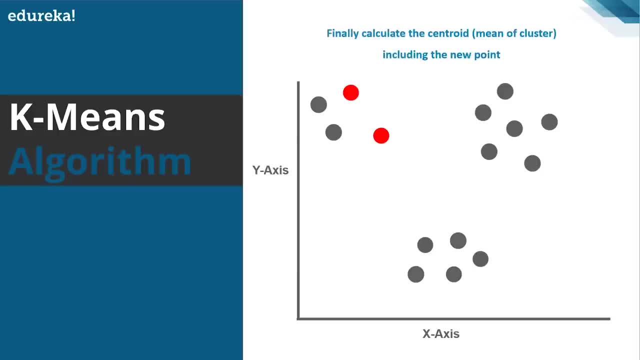 to the nearest cluster. finally, calculate the mean of the cluster with the new point in it, and we'll use this mean to determine the distance from the cluster. Yeah, we need to pick a bunch of starting points before finalizing the cluster. All right, now, coming to one of the most important question. 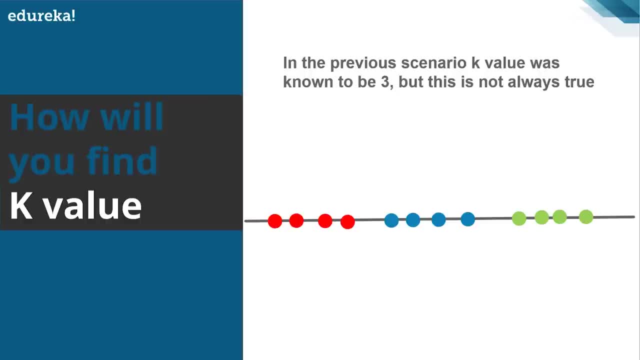 How will you decide what value should you use for K? Well, sometimes you will find that the number of cluster to create- obvious like K- equal 3, but sometimes it is not that easy to judge or guess the number of cluster manually. So what will you do in this case? 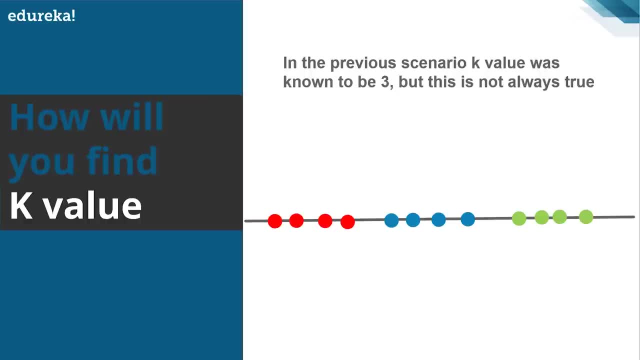 Well, one of the option to decide the value of K is a hit-and-trial method where you just need to try different values of K. So, starting with the minimum possible value of K, that is, K equal 1 of, it symbolizes that all the data points lie within one single cluster, K. 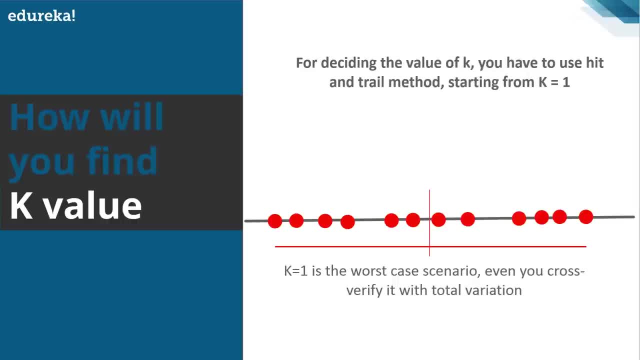 equal 1 is the worst case scenario. You can even decide it by calculating It's total variance. All right, by this what I mean to say? suppose you have 20 data points or late and you are creating 20 cluster. So this would be the worst case scenario. 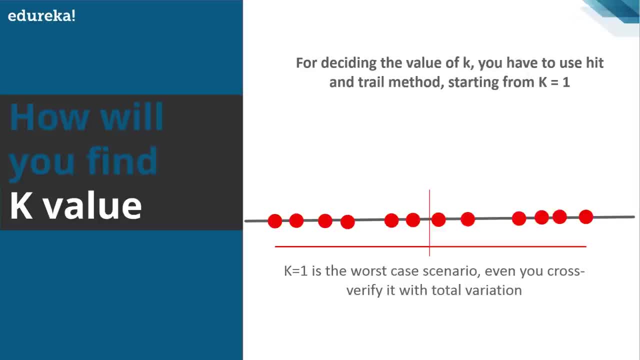 if all the 20 points are lying within the 20 different cluster. All right, Now let's try with K equal to- still better. But how much better will? why don't you compare it with the total variation, with K equal 2 to K equal 1? 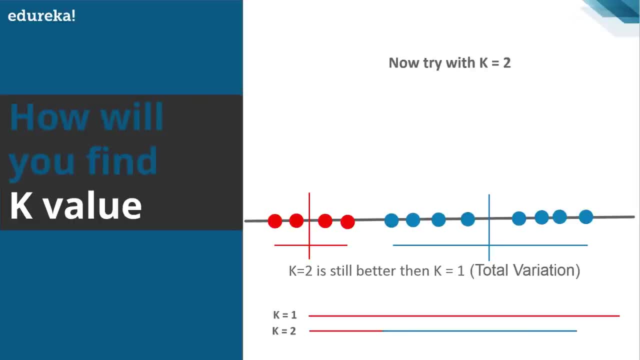 that is compared when we had two cluster to when we had one. Now let's try: K equal 3.. Well, in this case it's even better. But how much better will even in this case? you can decide it by comparing the total variation. 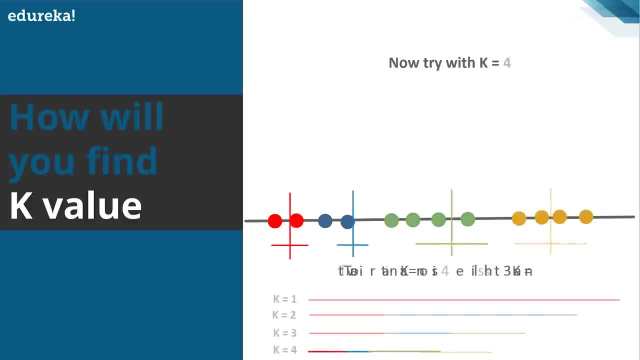 within the three cluster, that of the two. Okay, now try with K equal 4. in this case, that total variation within each cluster is less than when K equal 3. each time we increase the number of cluster, the total variation within each cluster gets smaller than before. 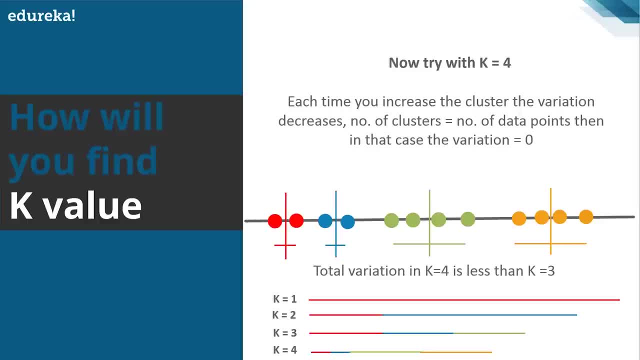 and then, finally, when we have the case where total number of cluster equal total number of points, or in other words we have just one point per cluster, Then in that case the variation becomes 0. obviously right. so you can say that the number of clusters are indirectly proportional. 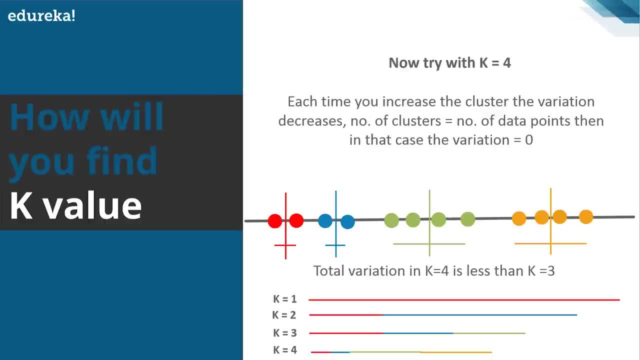 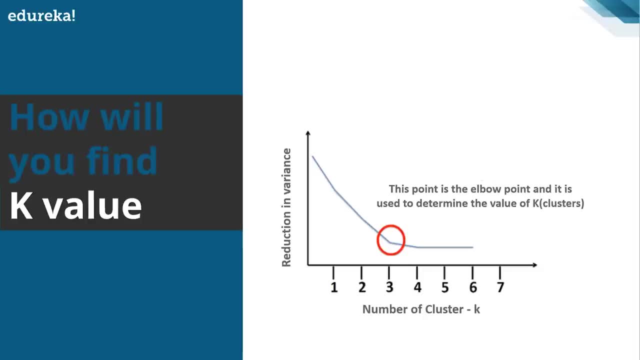 to total variation. if the number of cluster increases, the total variation decreases. finally, when we plot the reduction in variance for per value of K will get a graph like this, where on the x-axis We have the number of cluster K and on the y-axis we have reduction in variance. 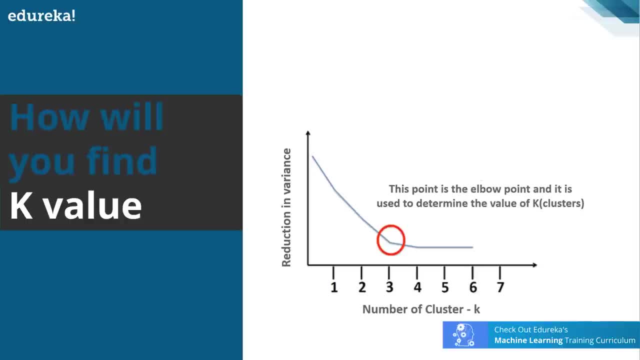 on the graph you can see that there's a huge reduction in variance, with K equal 3, but after that there is no such steep change in the variation. So this point of change is known as the elbow point, and the value of this point is the one. 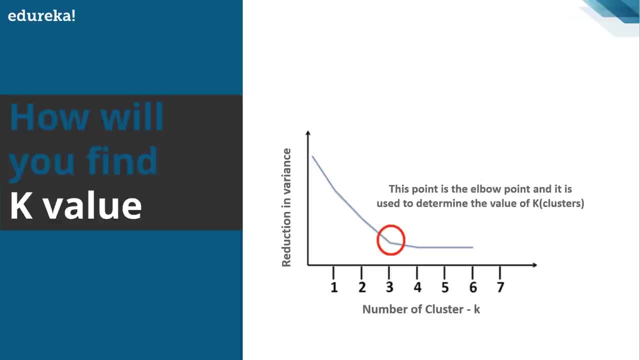 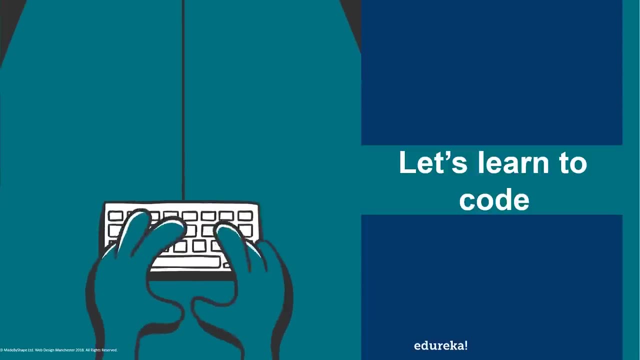 which decides the value of K. that is, in order to find out the value of K, You need to find the elbow from the elbow plot. Okay, fine, This was all about k-means algorithm, how it works. All right, Now let's move to the coding part. 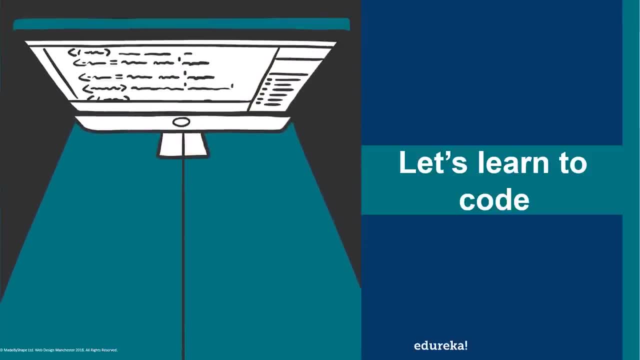 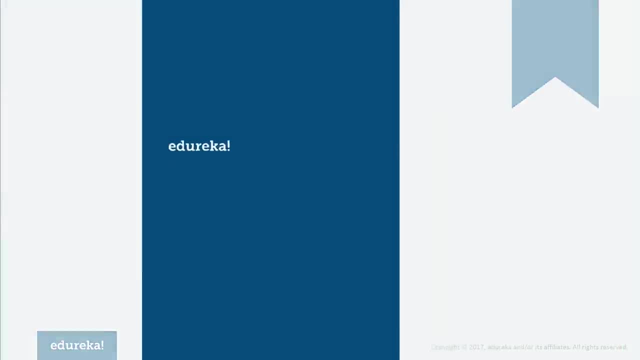 But before we dive into it, let's understand the algorithm on the basis of the coding. Let's move towards the implementation part of k-means using Python. But before that, let me just summarize the algorithm for you. Okay, So what we do? initially, we randomly choose K examples. 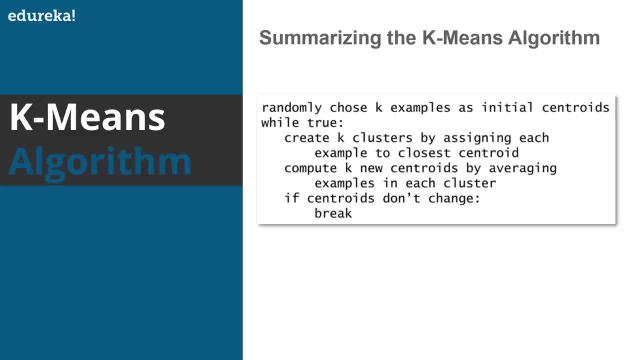 as initial centroid and, while true, we create K clusters by assigning each example to the closest centroid. So, first of all, what we do? we randomly choose K examples as initial centroids, then we check the condition. while true, then what we have to do in that case, unless and until it is. 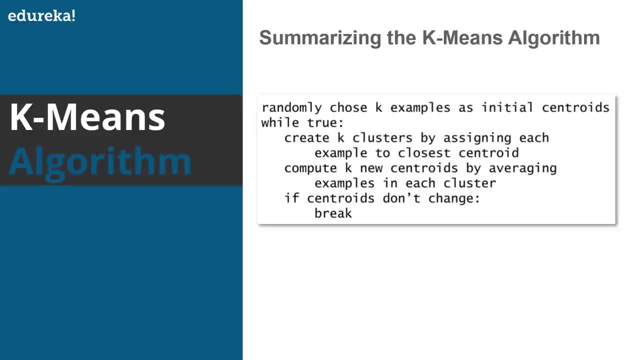 true will be creating K different cluster by assigning each example to the closest centroid, and then we'll be computing K new centroids by averaging examples in the cluster, and if the centroid doesn't change, that means we have found the exact number of clusters, All right, and then break the thing. 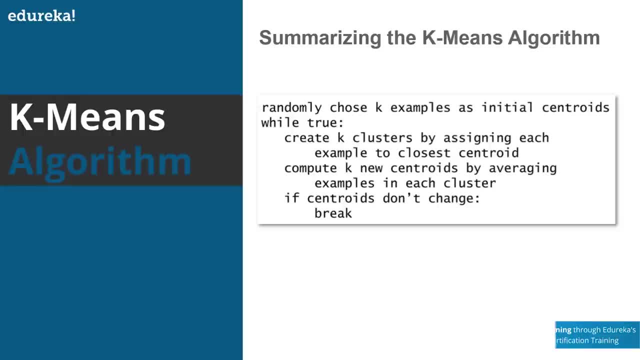 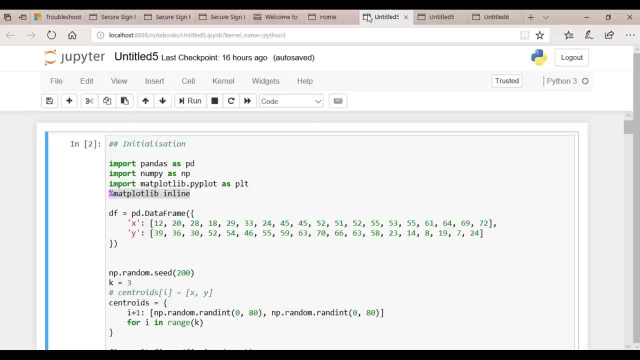 So this was a summary of k-means algorithm. Now let's move on to the implementation part. Let's see how to implement k-means clustering algorithm in Python. So in the first step, what you'll do? you will be importing all the important modules, such as Panda, numpy, sklearn. 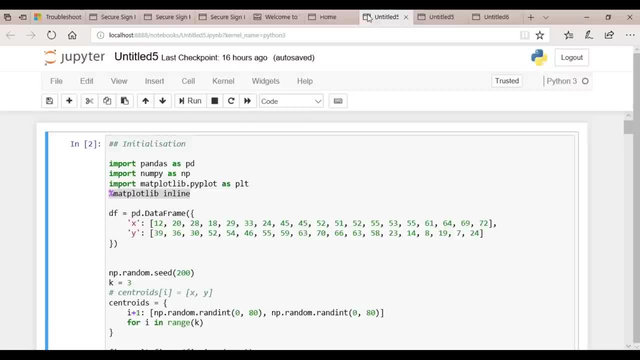 and pi plot. and the next step: you'll be importing the iris data set into the python, which is a very standard data set for classification problems and can be downloaded from the UCI repositories. in the third part You'll view the data set, study it. 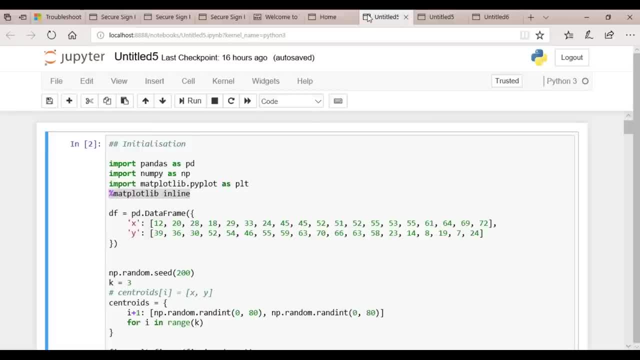 and then convert the data set into Panda data frame. All right, as a step, for finally will perform the k-means analysis on it and see the result of the cluster as a cluster vector and also as a plot. All right, and then, finally, we'll be using a python library. 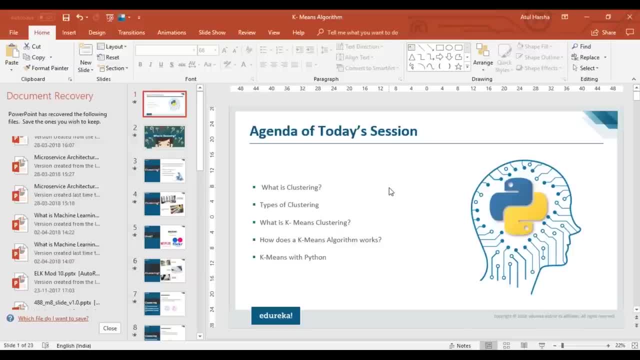 to implement the k-means clustering. Let's see how to implement k-means clustering algorithm in Python. So for this we'll be using two methods. The first method would be writing a k-means clustering program from the scratch, and the next method would be: 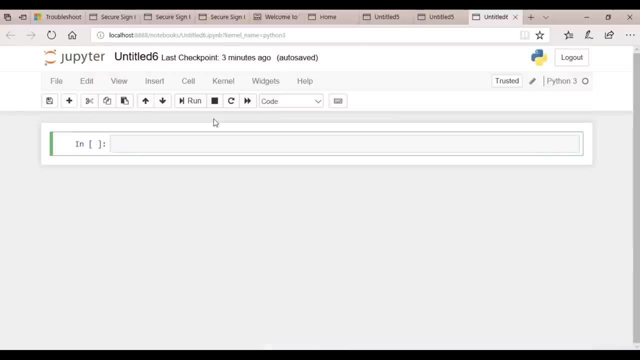 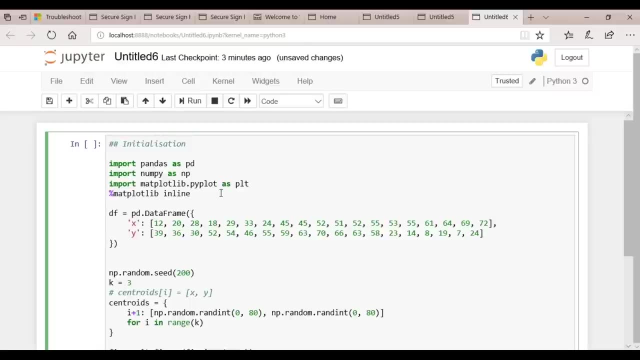 using a python library- sklearn. So our first part in this implementation would be the initialization part, and how it is will start by importing pandas, numpy and matplotlib. All right. next we'll define a panda data frame variable. DF says that the x coordinates are this and the y coordinates are this. all right next. 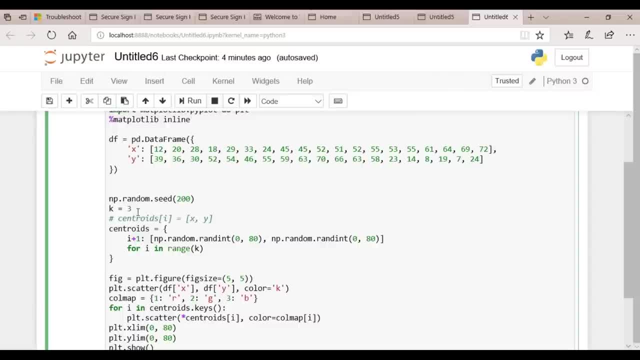 what we are doing. We are defining a random seed as 200 and defining K for the k-means clustering, or the total number of cluster that we want is 3.. The next task is choosing the first centroid. All right, fine. So these numbers lie between 1 to 80, right? 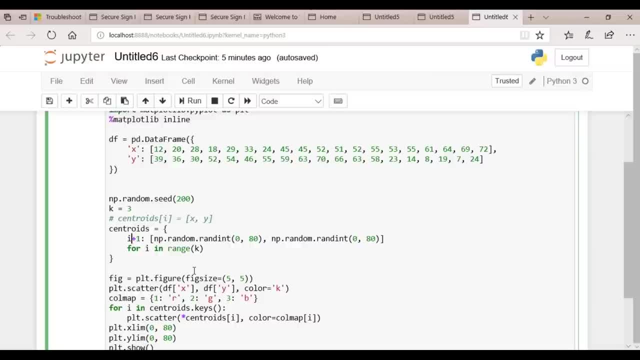 So for choosing centroid, I'll be using any random number between 0 to 80. fine, So here, plot dot, scatter. what we are doing here? We are creating a scatter plot such that on x-axis there will be data frame with the x-array. 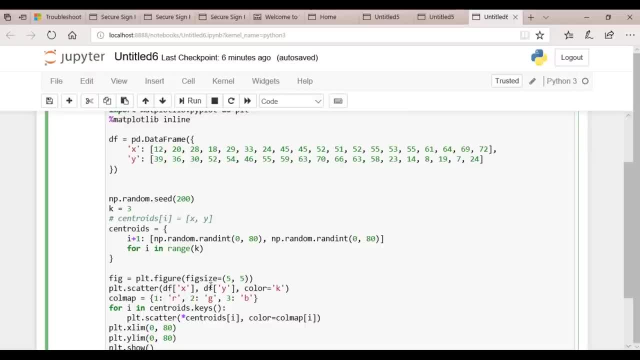 We are passing this value of x-array into the data frame and next we are passing the value of y in the data frame and we are defining color equals 3.. That means we need three different colors as the number of K That is equal to 3.. 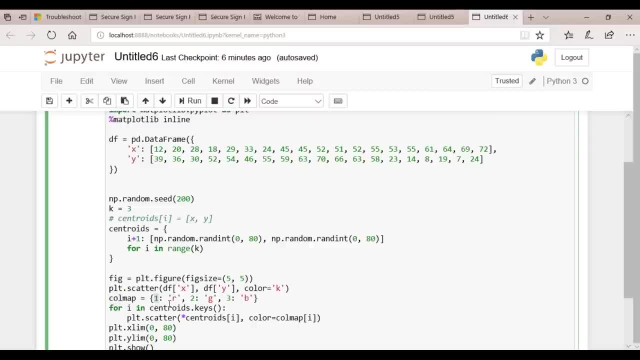 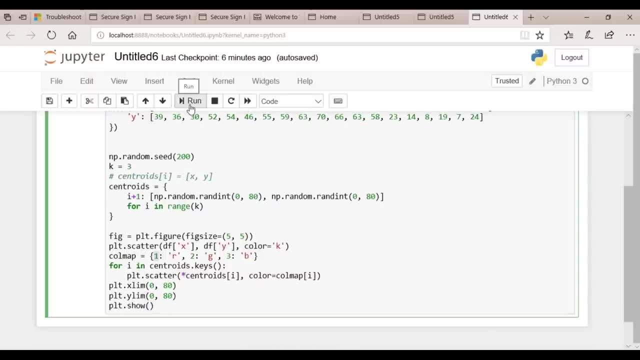 All right, as a color map, We are defining one for red, 2 for green and 3 for blue. All right, and finally, we are plotting it. Let's execute it and see what is the result. we are getting. Okay, this star mark. it symbolizes. 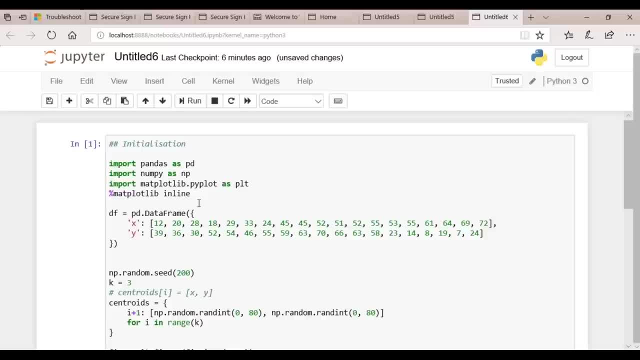 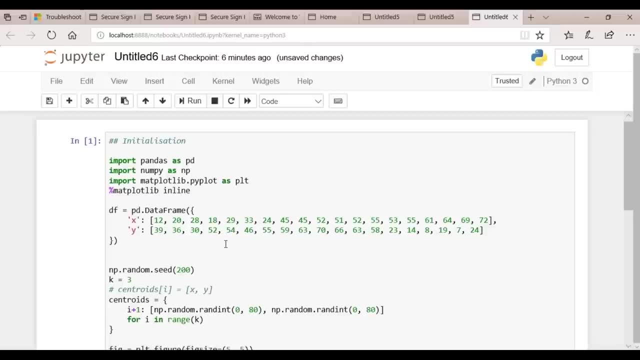 that it is still executing and once it will change to a numeric number- Yeah, like it turned to one, so it suggests that it has completed the execution and output is ready. Okay, so there's the output which you will get. you can see that this red green. 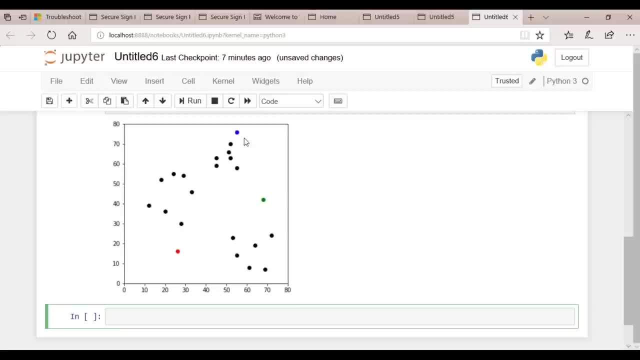 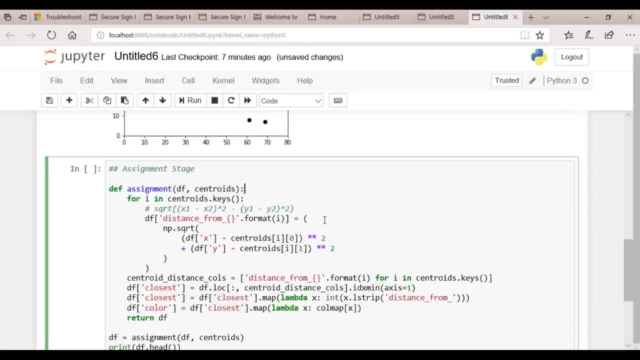 and blue are three random data points which are initially selected as the centroids. All right. Next is the assignment stage. I need to assign each point to one of the cluster. All right, So let's execute it and see a sample output of it. 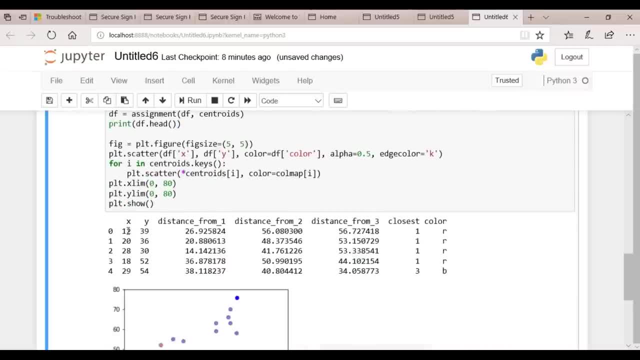 All right. So what we are getting here is that for the first point of coordinate 12 and 39, its distance from first cluster is 26.92, whereas its distance from second cluster is 56.08.. Well, in case of third cluster, it's 56.72.. 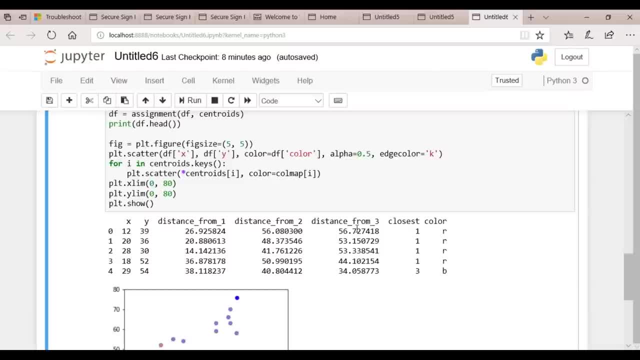 What we'll do will finally assign that point to that closest cluster, All right, which is 26 in this case. So the closest cluster is one, and we have already defined the color scheme for one was red, Okay. similarly for the second point, third point, fourth, fifth. 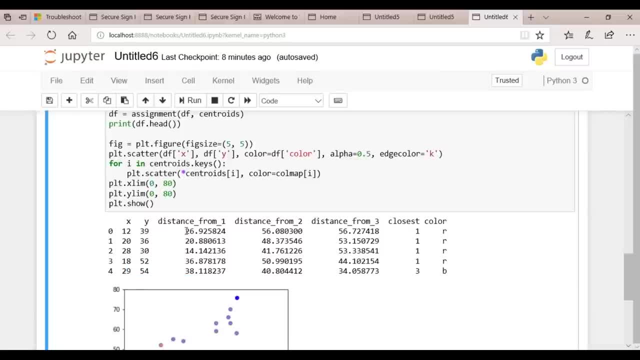 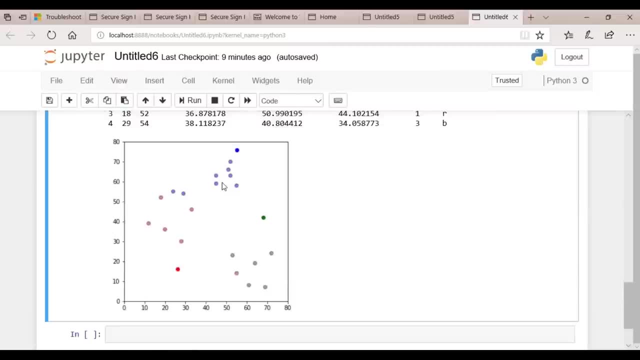 and so on. All right, what we have to do? We have to check the distance from first, second and third cluster. whichever is the minimum will assign that particular point to that particular cluster. All right, so this is done. So next is the update stage. 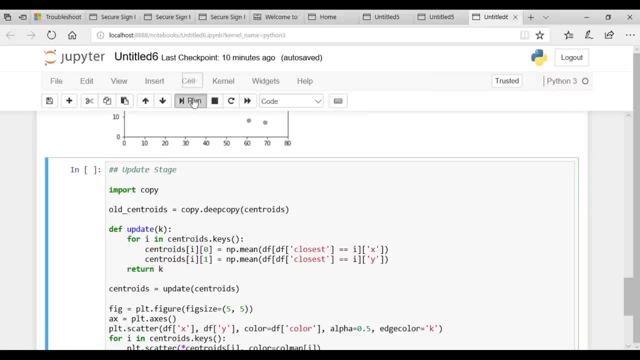 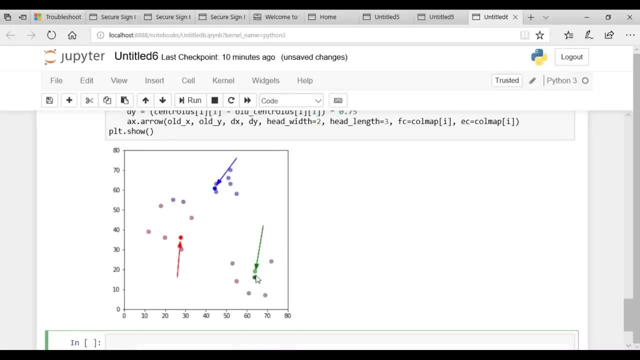 where the centroids will be updated. All right, so let's execute it and see. you can see that these are the updated centroids. the centroid are shifted somewhere in the middle of the screen cluster. All right, so this update stage what it did? It just updated the value of the centroid such 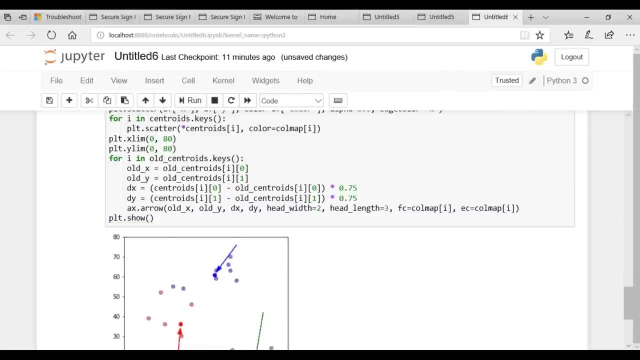 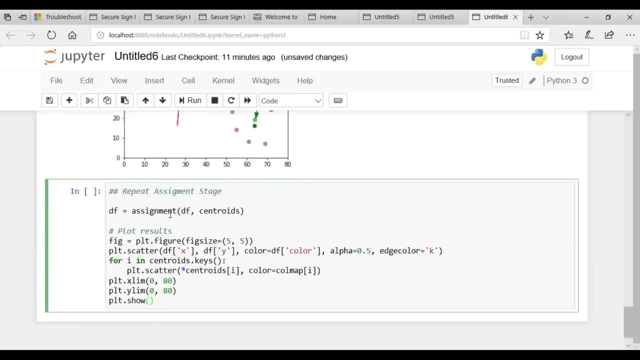 that it lies somewhere between the cluster. All right, Okay, Now this is done. Then what we have to do is we have to again define the assignment stage. So we'll define a DA variable consisting of assignment function and that will pass a value. 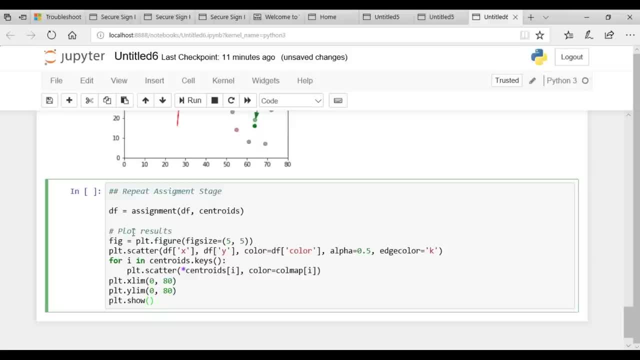 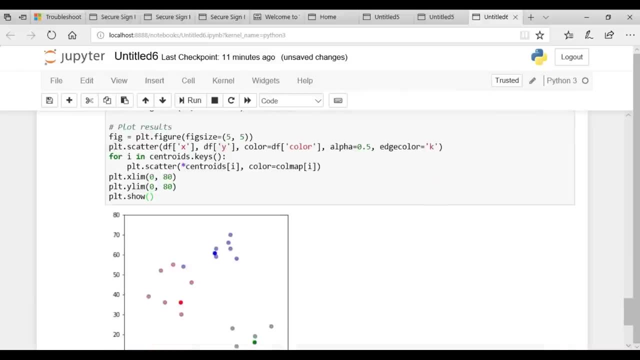 of ponder data frame and the centroids, All right, and then again we'll plot this result. Okay, let's see how it shows. Okay, let's compare these two result. Are you getting any difference? Yeah, you can see that. this particular blue point. 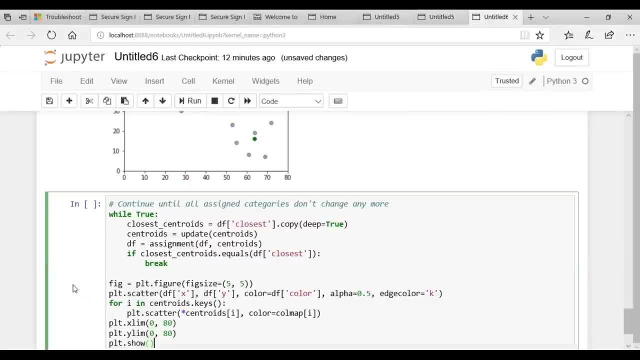 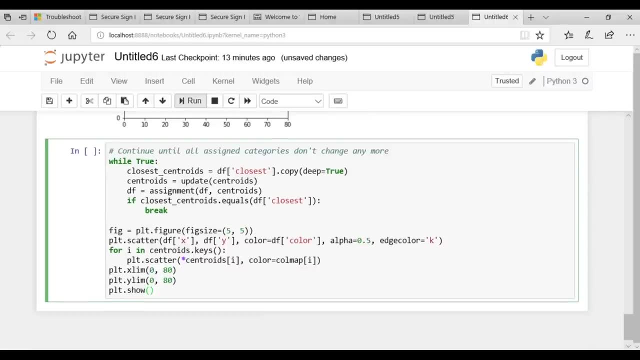 is changing to red in this graph, right, Okay, Now this process will keep on repeating until and unless all the assigned categories does not change anymore. All right, let's execute it and see. Okay, so let's compare the two result. 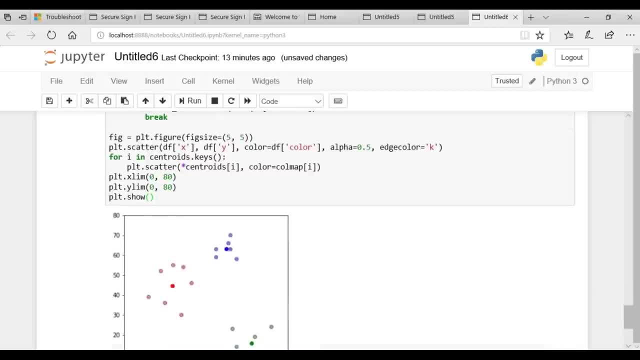 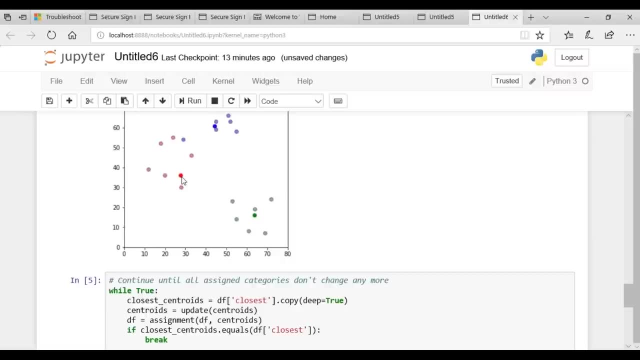 Okay, even in this case, this blue- This is changed to red And our centroid, which was initially positioned here, is changed to somewhere in the center of the cluster. All right, So this is our final result and we have three clear cluster with three means. 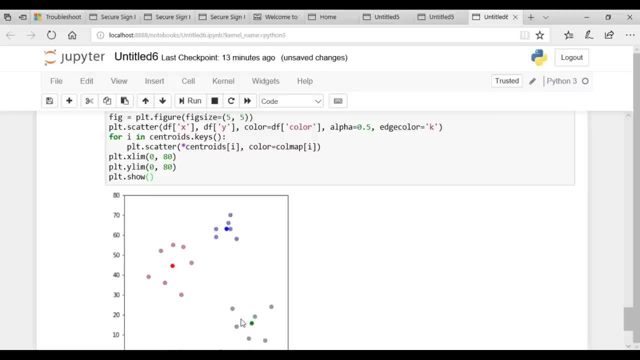 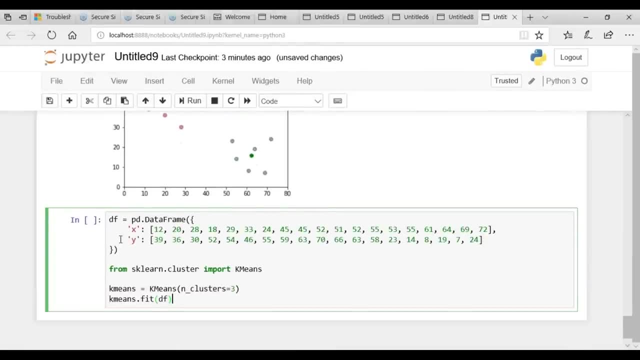 at the center of these cluster. Now let's repeat the same task using this cyclic learn. We first fit to our data, So for that Let's see Fine. Next what we'll do: we'll Define the data frames. Let's load our data and Define the k-means. 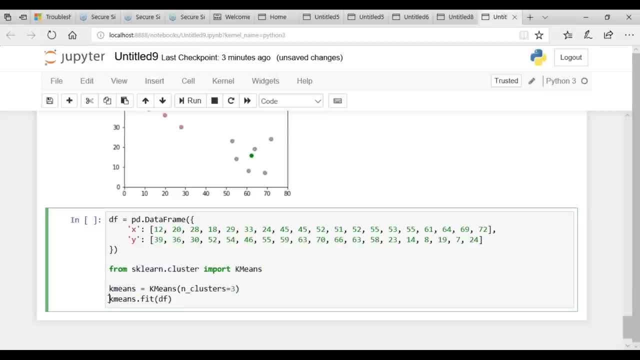 and k-means will be Defining the total number of cluster as three. All right, So here what we are doing: We are creating a variable for ponder data frame, which will be storing the values of x and y coordinates. All right, then, from sklearncluster will be importing the k-means. 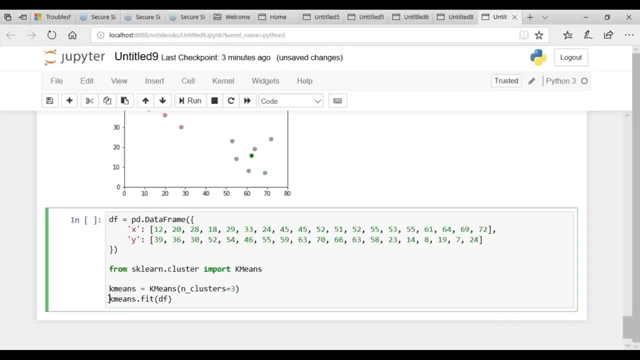 k-means is a predefined library which comes under the sklearn. We'll Define the total number of cluster for k-means and then, finally, we will fit our data to it. All right, let's execute it. Okay, So there's our output. the algorithm is Auto copy.